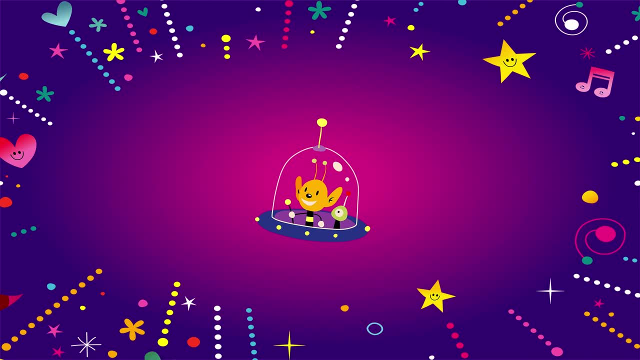 Now we're going to play a little game with our breathing. It's called space breathing. We're going to leave a bit of space after each breath out Before we breathe in again. To make it work, we count silently after each breath out, before we breathe in. 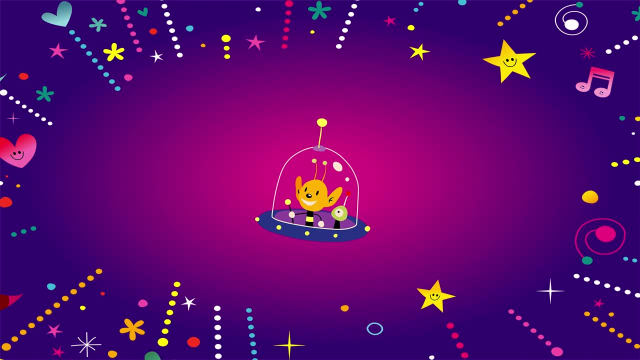 We start with a count of one, then one, two, right up to a count of seven. Now don't worry if the count of seven seems too much. You can always breathe whenever you need and you must. This is about you feeling comfortable and relaxed. 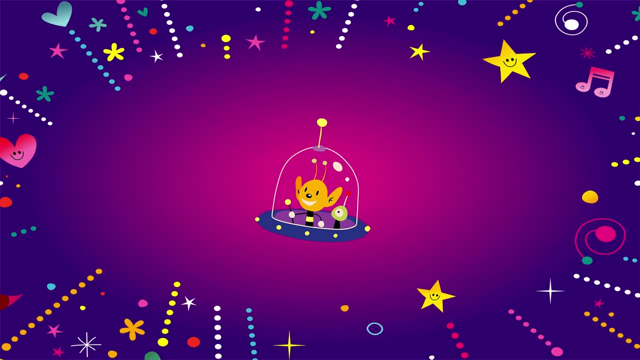 So just see, Listen to your body. There is no winning or losing in this game, Only playing. Okay, Let's begin by tuning into our breath again, So we're ready. Notice it quietly coming in and going out, Coming in. 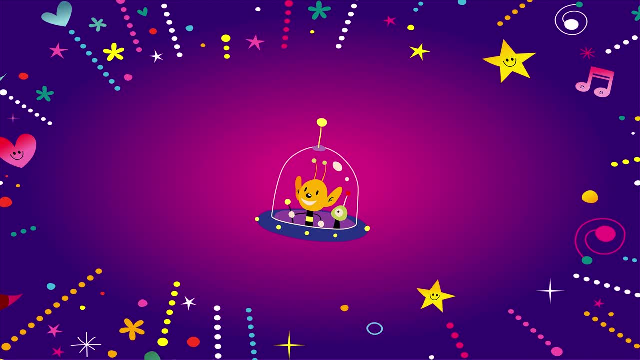 And going out, Not holding it, Just letting it flow Calmly and steadily Without you doing anything. This time, after your breath out, count one. Then breathe in again After the next breath out, count two: One. 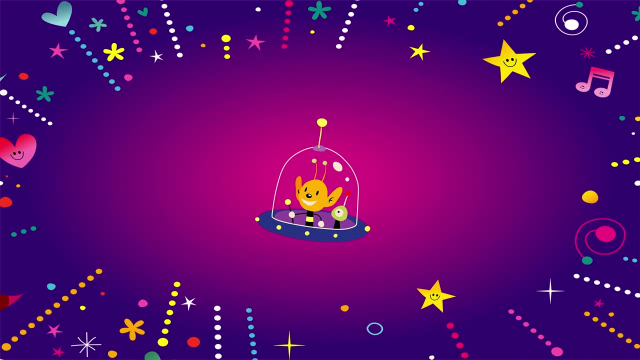 Breathe in One, Two, Three, Four, Five, Four, Five, Six, Seven, Eight, Nine, Ten, Eleven, Twelve, Three, Four, Five, Eight, Seven, Nine, Ten, Twelve, Three. 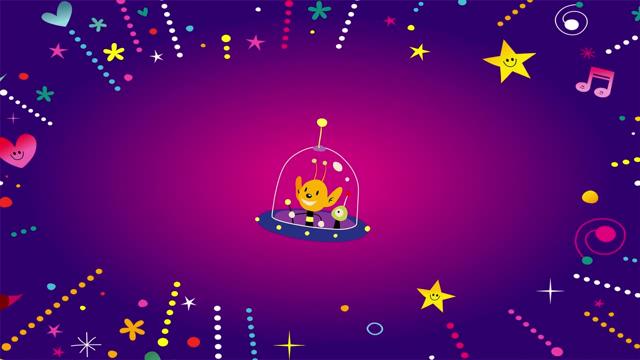 Four, Four, Five, Eight, Nine, Ten, Twelve, now out count six, Breathing in, and out count seven. Calm and easy breathe. if you need to Just allow the space to be there After reaching seven, allow your breath to come back.